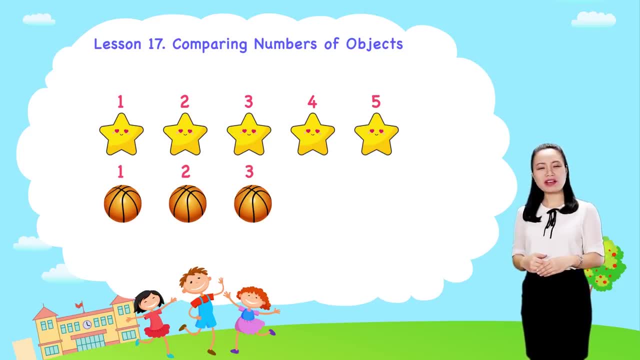 If we pair a star with a ball, then two stars are unpaired, because there are more stars than balls or there are fewer balls than stars. So we say the number of stars is more than the number of balls, or the number of balls is less than the number of stars. 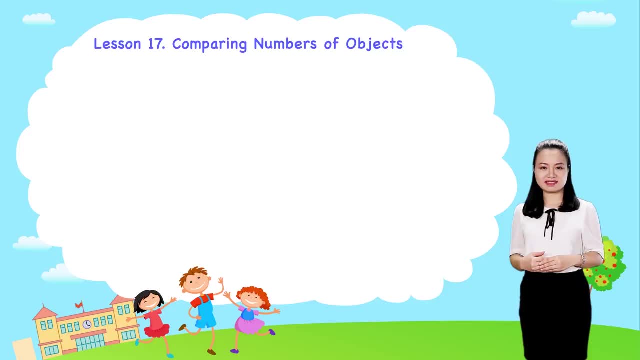 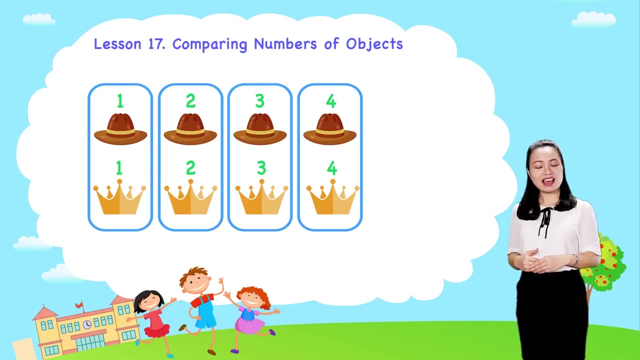 Next, We have 4 hearts and 4 crowns. If we pair a heart with a crown, then each heart is paired with a crown because there is an equal number of hearts and crowns. So we say the number of hearts is equal to the number of crowns, or the number of crowns is equal to the number of hearts. If we pair a star with a ball, then two stars are unpaired, because there are more stars than balls or there are fewer balls than stars. If we pair a star with a ball, then two stars are unpaired, because there are more stars than balls or there are fewer balls than stars. If we pair a star with a ball, then two stars are unpaired, because there are more stars than balls, or there are fewer balls than stars. If we pair a star with a ball, then two stars are unpaired because there are fewer balls than stars. 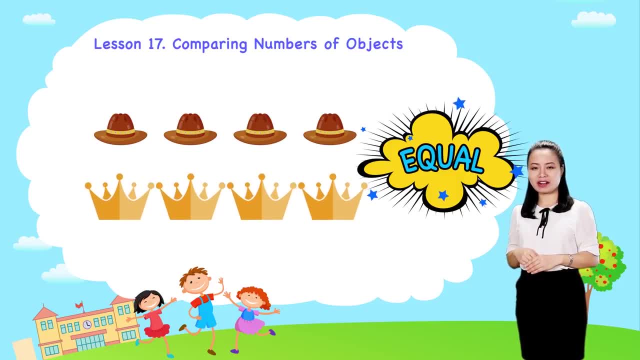 If we pair a star with a ball, then two stars are unpaired because there are fewer balls than stars. If we pair a star with a ball, then two stars are unpaired because there are fewer balls than stars. number of crowds, or the number of crowds is equal to the number of hearts. I hope. 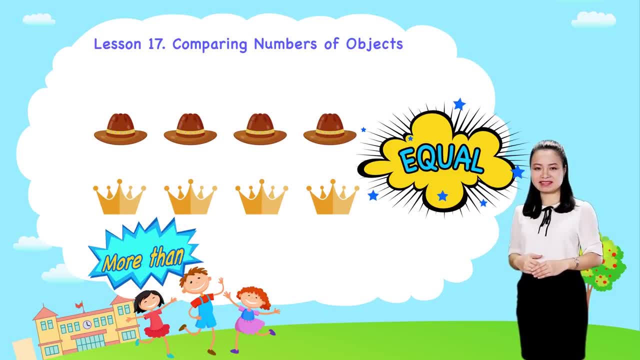 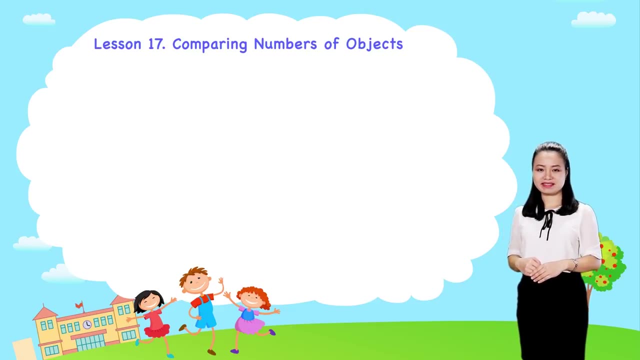 you understand more than less than or equal to. now let's have some practice. look, we have six apples and four bananas. look, we have six apples and four bananas. look, we have six apples and four bananas. is the number of apples more than less? is the number of apples more than less? 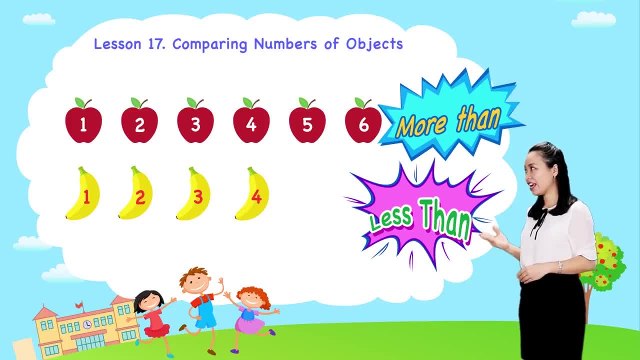 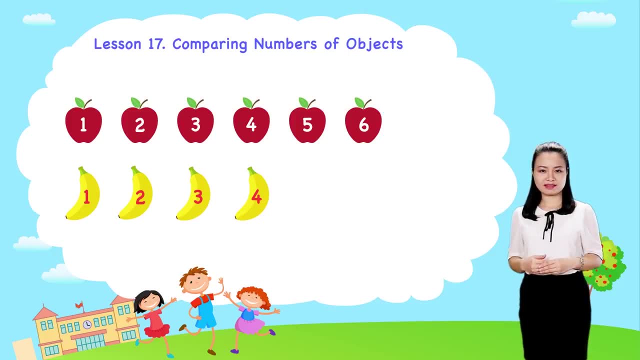 is the number of apples more than less than or equal to the number of bananas, than or equal to the number of bananas than or equal to the number of bananas. let's have an apple with a banana, then let's have an apple with a banana. then let's have an apple with a banana, then two apples. 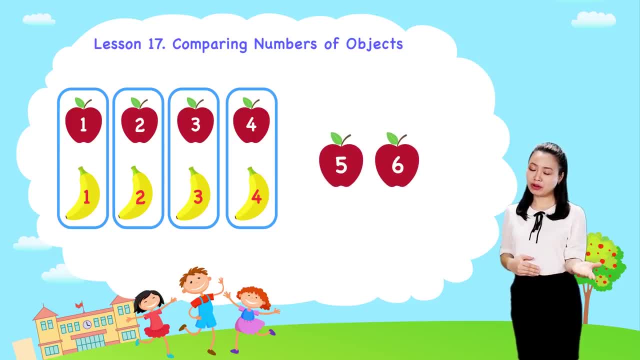 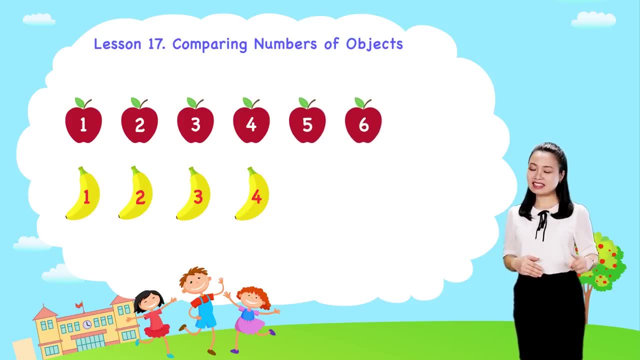 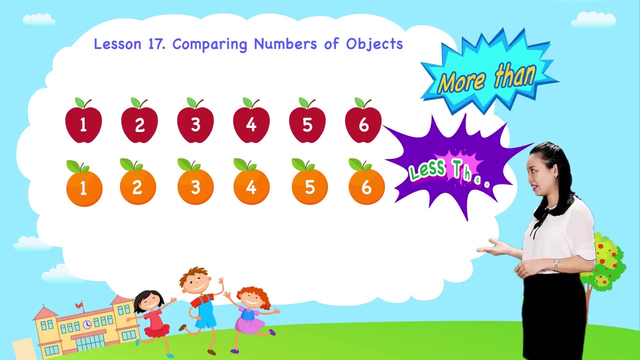 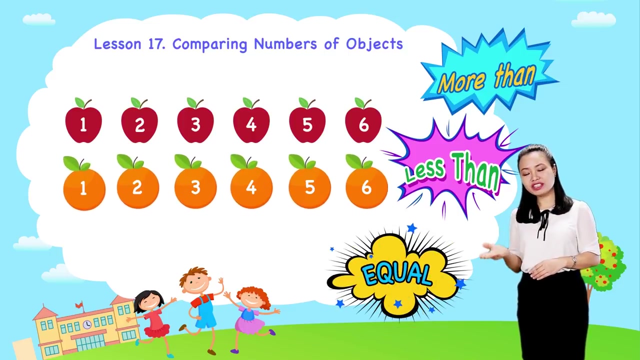 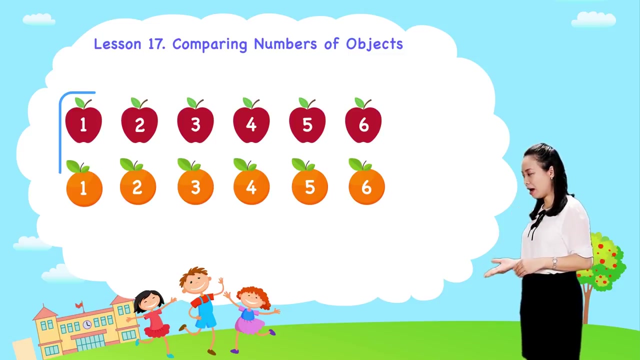 two apples. two apples are unpaired because there are more apples than bananas. so the number of apples is more than the number of bananas. next we have six oranges. is the number of apples more than, less than or equal to more than less than or equal to the number of oranges? let's pair an apple with an orange, then each apple is. 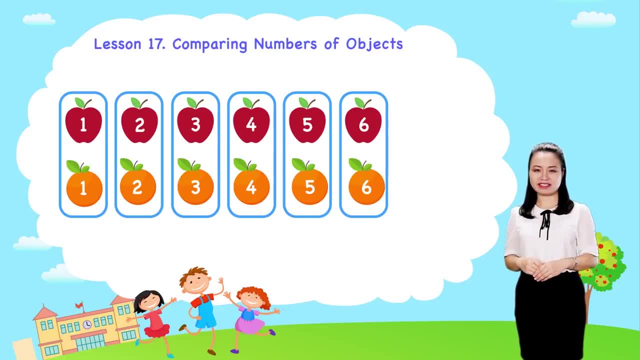 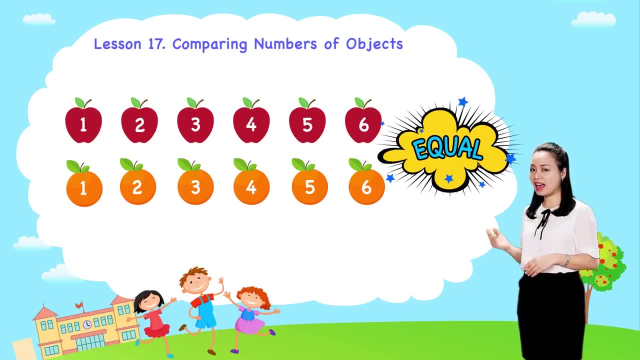 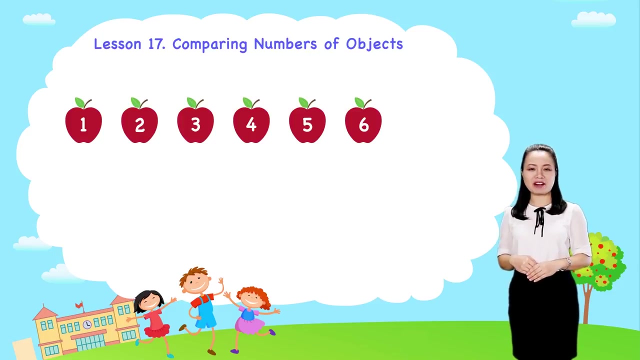 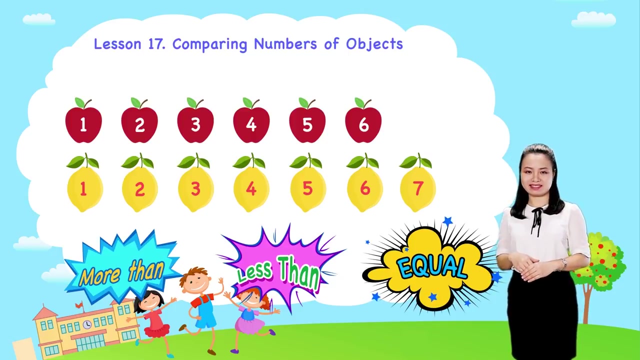 paired with an orange, because there is an equal number of apples and oranges. so the number of apples is equal to the number of oranges. next we have seven lemons. is the number of apples more than, less than or equal to the number of lemons? let's pair an apple. 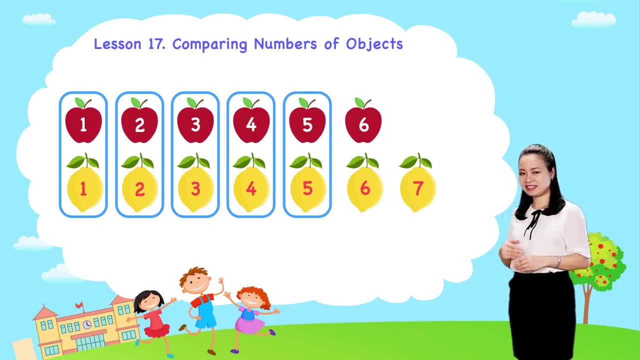 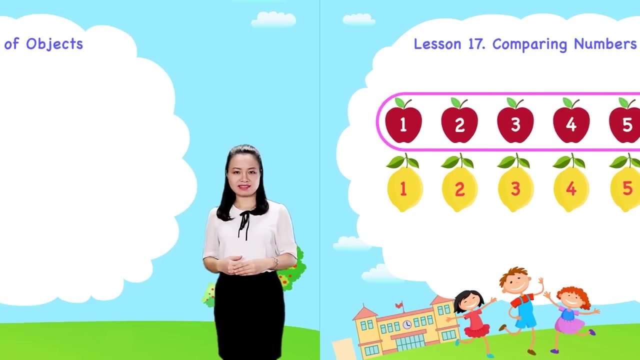 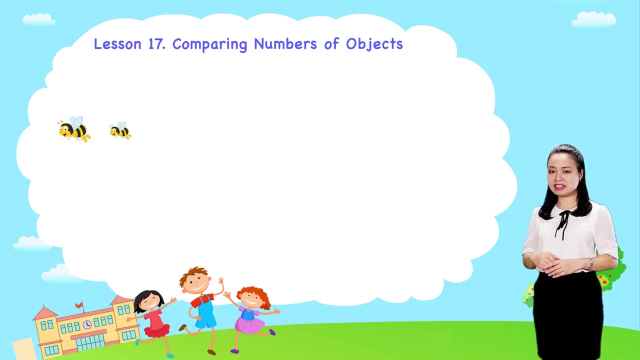 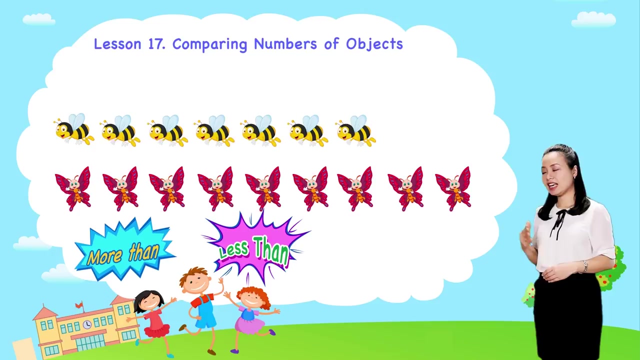 with an apple, with a lemon, then one lemon is unpaired because there are fewer apples than lemons. so the number of apples is less than the number of lemons. now we have a number of bees and butterflies. is the number of bees more than, less than or equal to the number of butterflies? 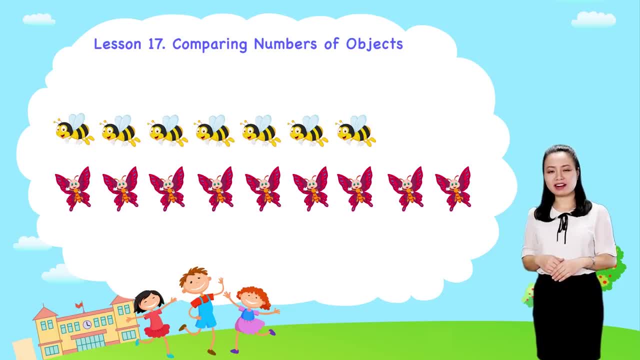 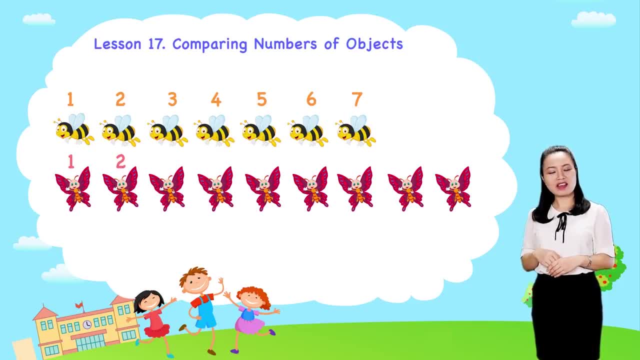 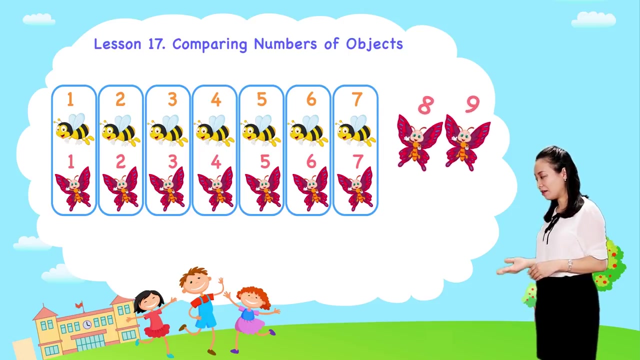 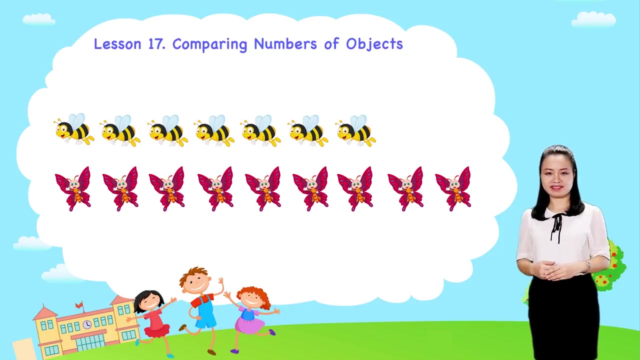 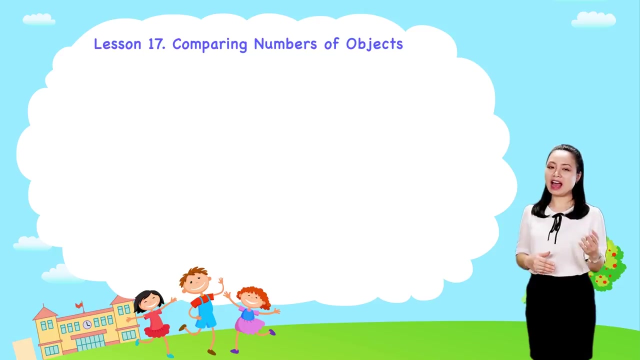 one, two, three, four, five, six, seven, eight, nine. let's pair a bee with a butterfly, then two butterflies are unpaired because there are fewer bees than butterflies. so the number of bees is less than the number of butterflies. now we have a number of pigs and chickens. is the number of pigs more than less than?